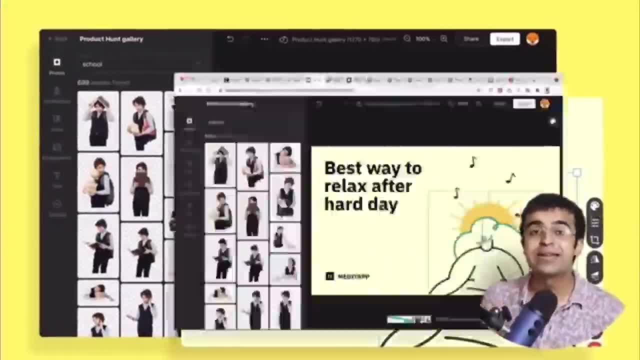 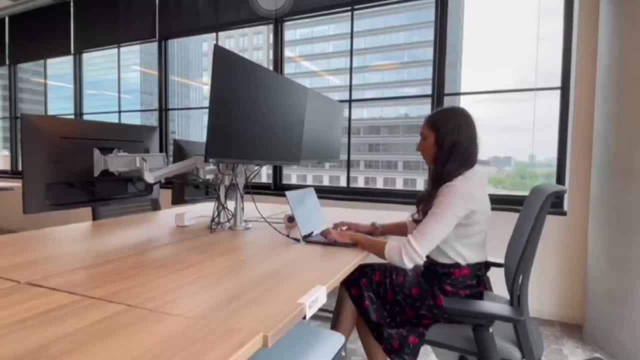 games and colorful UIs. I didn't really understand all the hype around the fundamentals. Eventually I did what any other struggling college student would do when they weren't really doing well in class: I started going to TA sessions. Wait, TA sessions. I'm pretty sure you. 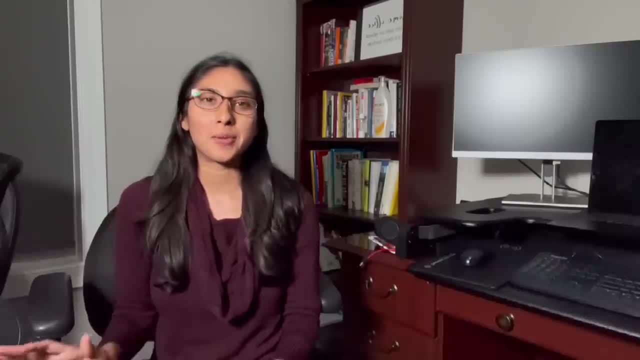 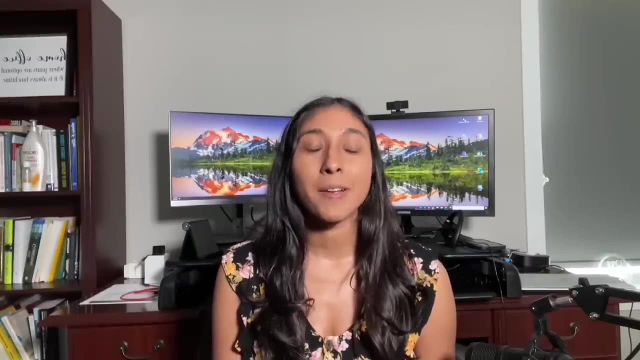 were blacked out drunk all of freshman year. There's no way you went to those, Uh yeah, Okay. so I did slack off a bit- my freshman year, I guess. But that came to bite me in the butt when I got my first C in chemistry. I quickly realized that the biomedical engineering 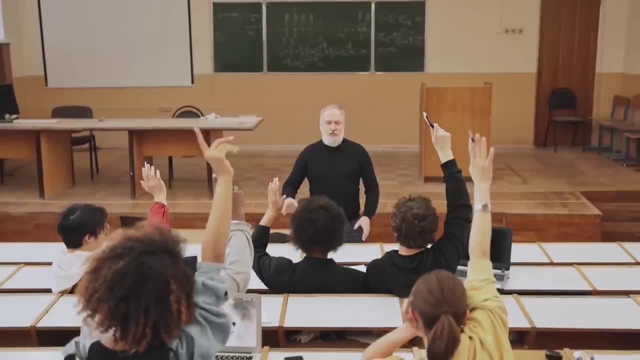 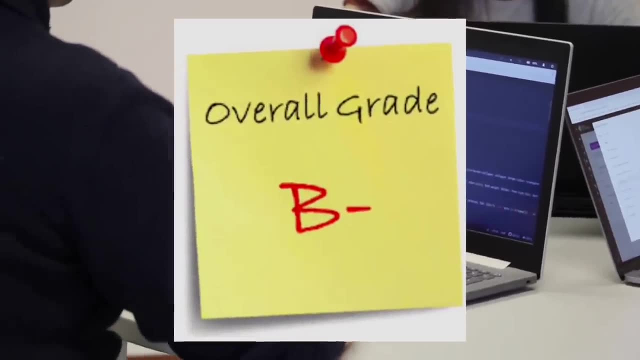 life wasn't for me. So I leaned back on the one coding class I took. Remember the Intro to Object Oriented Programming class I mentioned earlier? Well, yeah, I got a B- in it. So not great, but also not terrible for someone who put the bare minimum effort into classes that year. 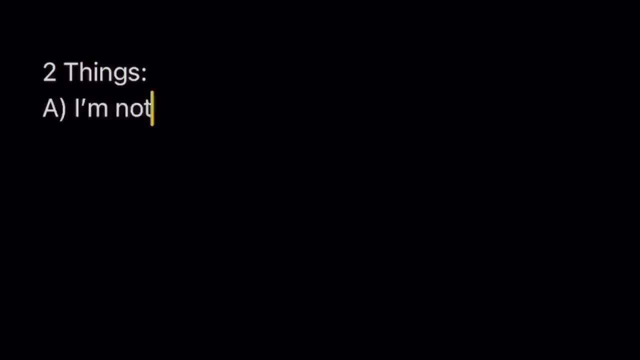 I quickly started to realize two things: A, I'm not that good at coding and B, I just want to survive getting through a computer science degree long enough to start making six figures. I know a very noble goal. So fast forward a bit to my sophomore. 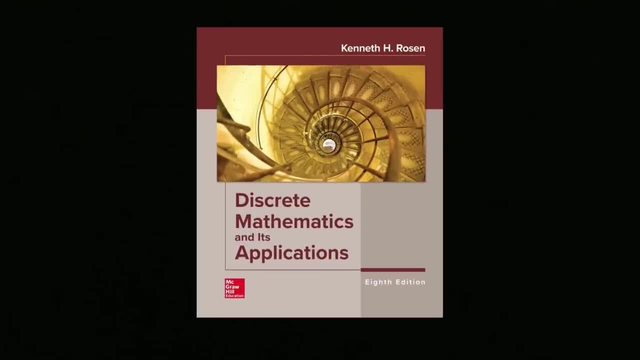 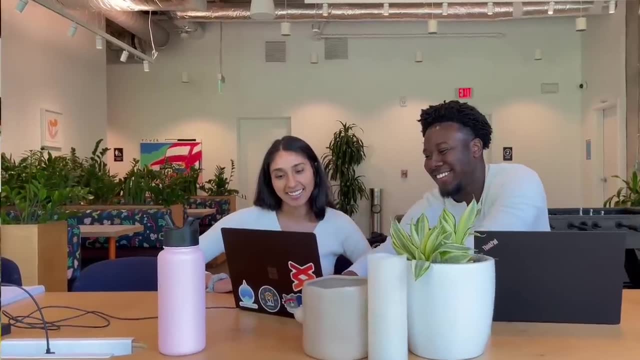 and junior years I was taking classes like discrete math, intro to algorithms and numerical analysis. I kind of glazed over those prerequisites but finally came alive during two classes. The first was data structures and algorithms. Now, if you're currently grinding, 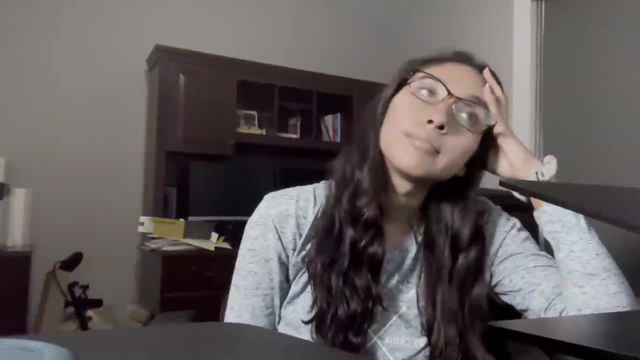 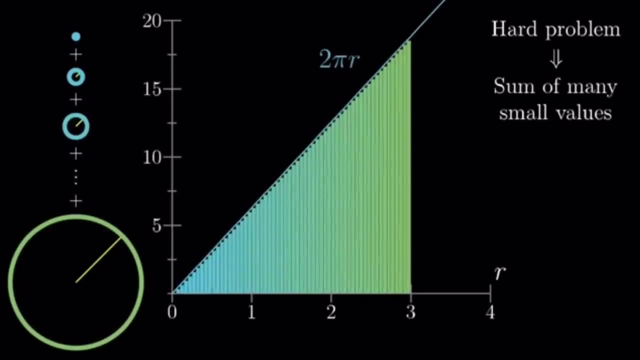 leetcode. you may have a slightly different view of data structures and algorithms, But for me it had a similar effect to calculus when I was first learning that Calculus was like a magic symphony that combined trigonometry, algebra, geometry and just basic arithmetic. 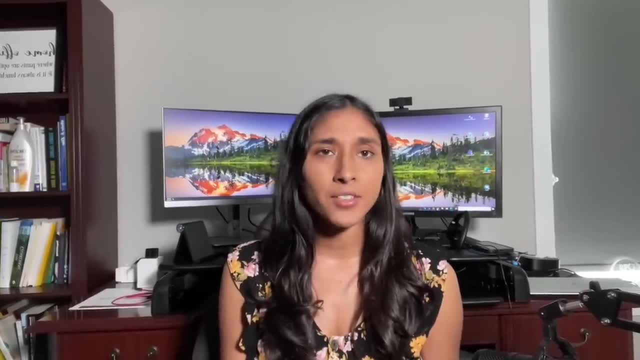 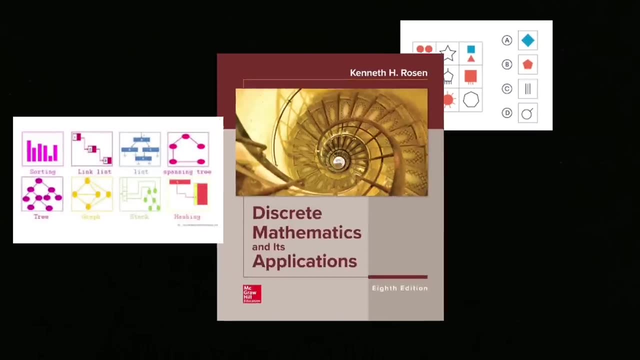 and spatial reasoning. Up until then, I had no idea why I was even learning about the properties of an obtuse or scalene triangle. Similarly, data structures, combined logical reasoning, discrete math and, yes, even the dreaded object-oriented programming into one beautiful 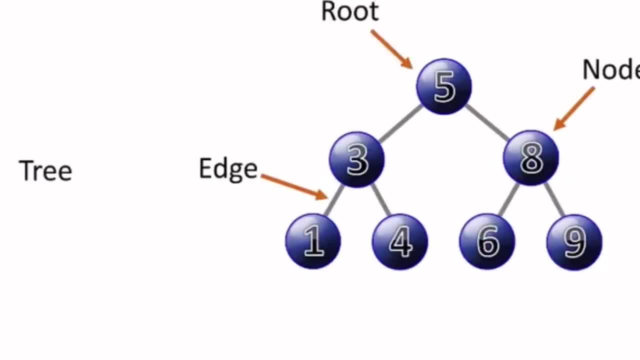 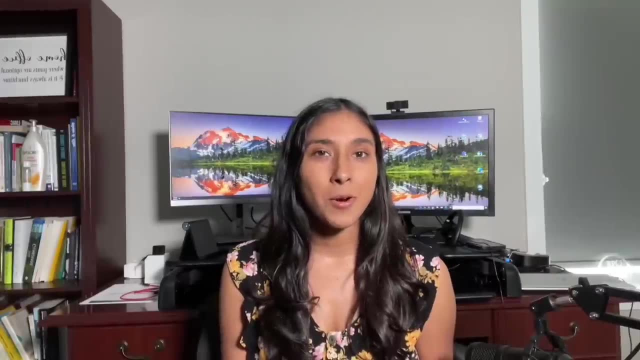 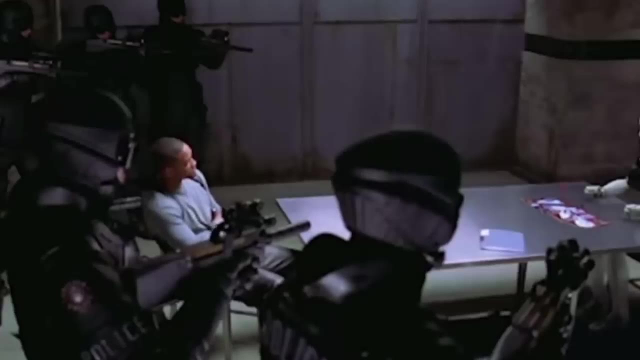 monolith. It finally started to become more fun to understand what a binary search tree was or even how to recurse through a graph structure using the A-star algorithm. Fast forward a bit more and I took another amazing class that sparked my interest: intro to artificial intelligence. Now, when you think of artificial intelligence, you may picture. 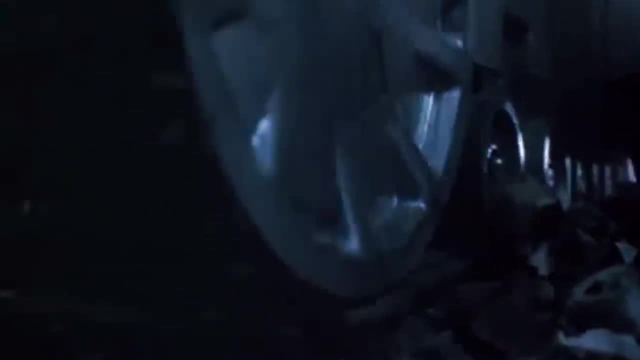 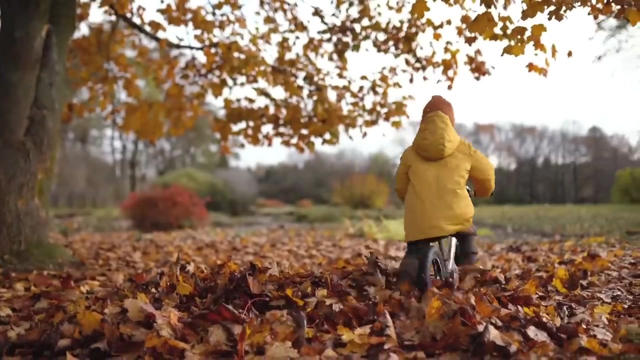 self-serving robots that annihilate humans off of the face of the earth, But in reality, they do pretty boring and mundane tasks by just adapting their functionality based on how a human would adapt their strategy when they learn something new. This is where I learned how to use neural 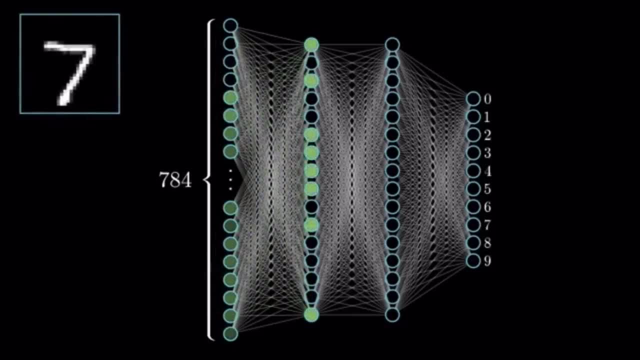 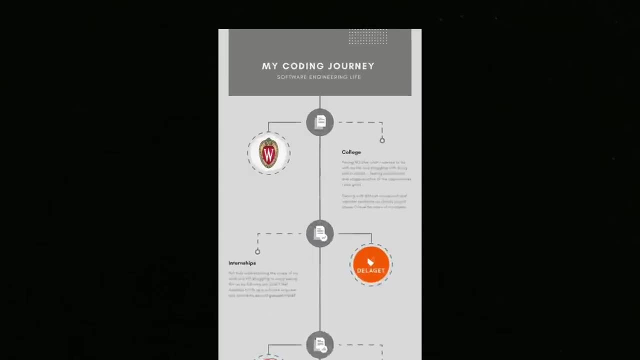 networks for pattern recognition and created a machine learning algorithm to play mancala against artificial intelligence. Spoiler alert: the computer beat me 99% of the time. I was feeling pretty good until I landed my first internship. The internship was at a small company. 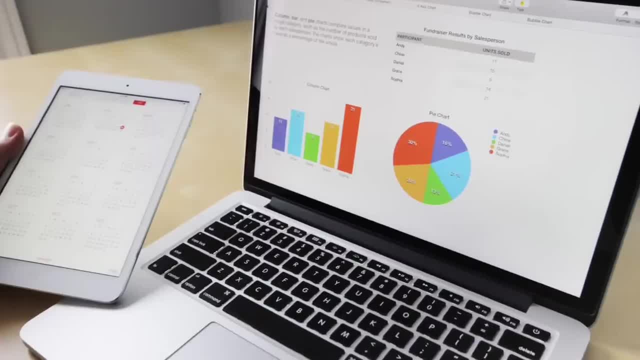 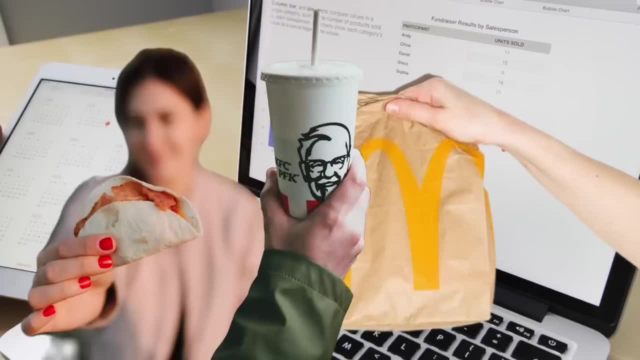 in Minnesota called Delegate. It was a fun summer. I created a tool to analyze employee and manager interactions at restaurants such as McDonald's, Taco Bell and KFC, But I had no clue what I was doing. I didn't really understand what razor code was and I mostly used C-sharp in the NET. 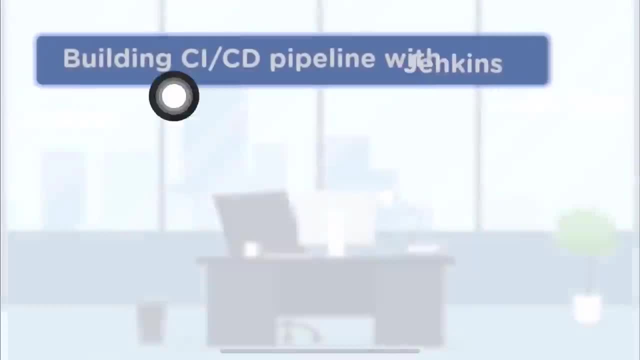 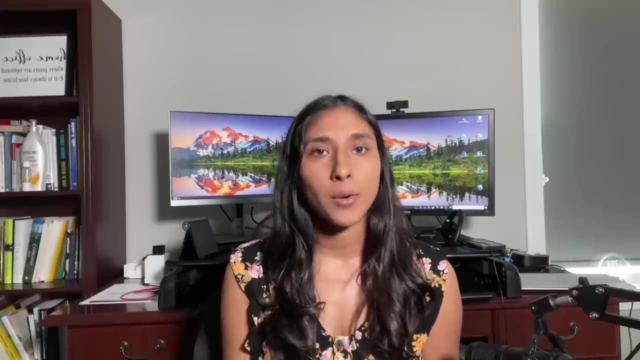 framework. This was the first time that I was introduced to concepts such as the CICD process, integrating unit and functional tests, agile methodology, as well as just understanding how to deploy code into the different environments and be versatile enough to take criticism when. 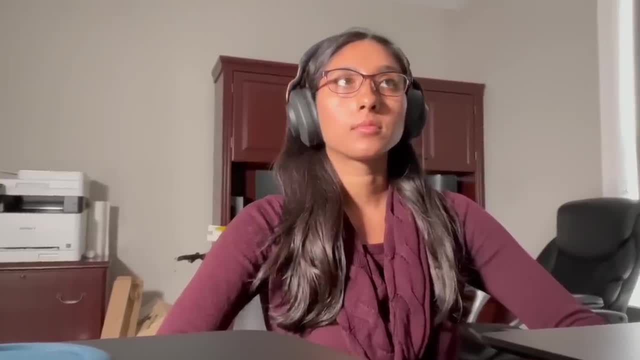 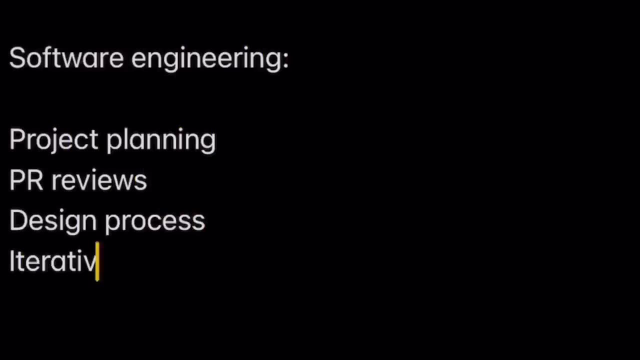 my code wasn't good. This was the start of understanding what it takes to be a software engineer. Being a software engineer meant way more than just coding. It meant understanding high-level abstractions of systems and knowing what to code and when. Anyways, back to the 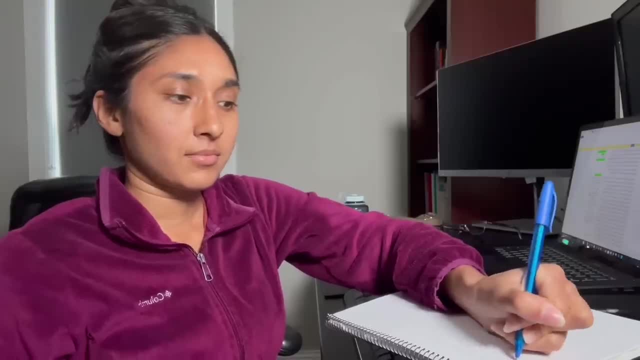 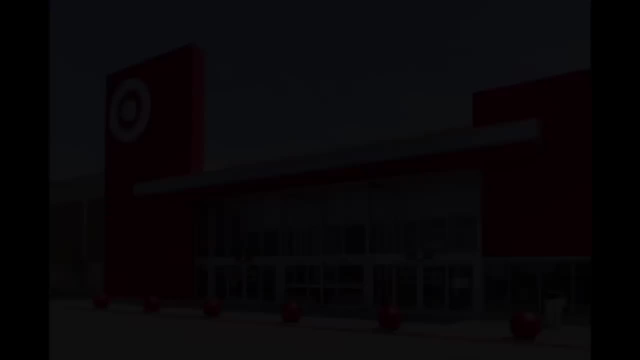 internship. I felt like I was being productive, yet I didn't have a deep understanding of what was going on. Essentially, I was just going through the motions. To be honest, I had applied to places like US Bank and Target whenever I would go to the career fair. 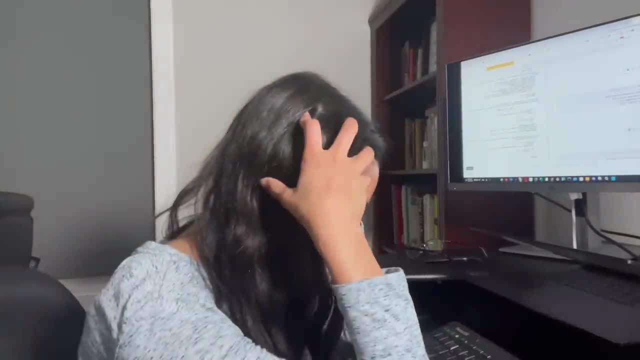 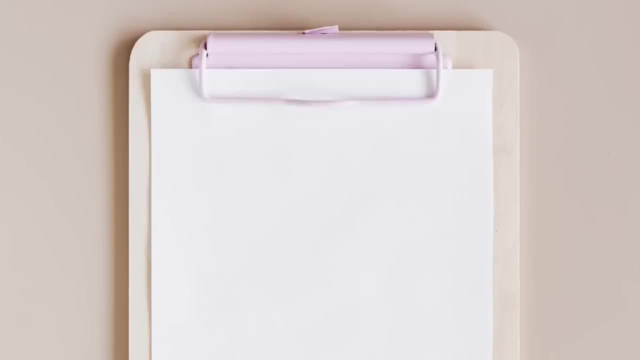 but I could never pass their interviews because I would get so much anxiety. when I was asked to code something in front of other people I felt like the interviewers were staring into my soul. I just never ended up doing that well to meet their bar And forget about applying to places. 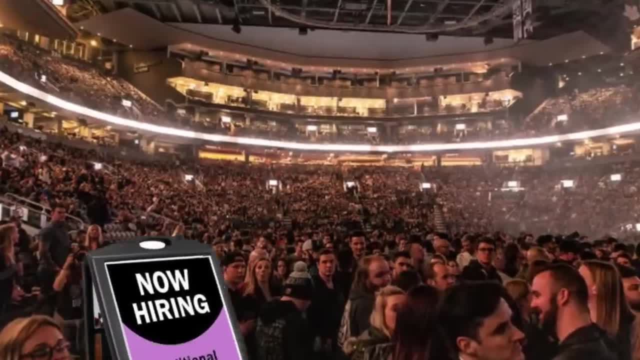 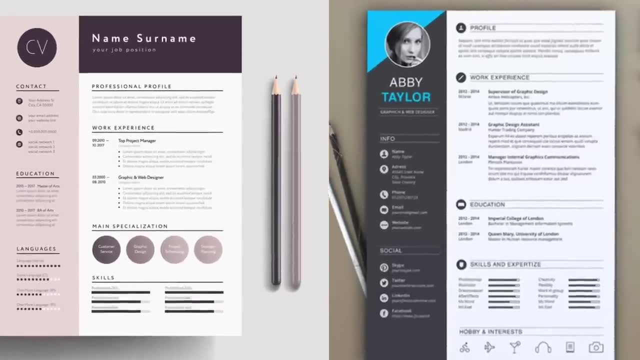 like Facebook, Google or Microsoft. The lines for these companies would always extend way past the entrance gate. I had no clue what I was doing and I didn't know what I was doing. I was just just an average B student that wanted to desperately secure a job, but there was no way. 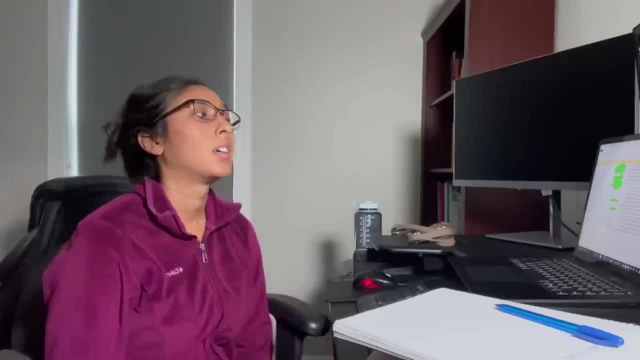 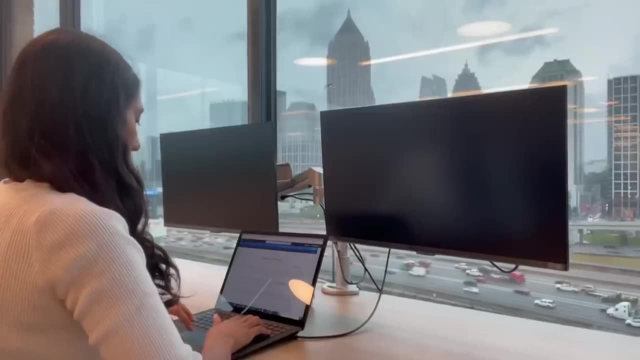 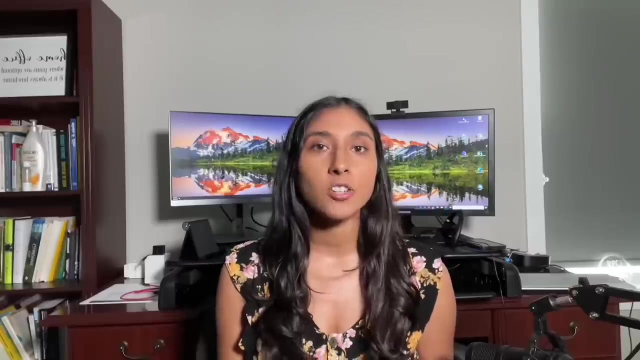 I could compete with those other students. I was feeling my lowest, as I imagined that I would never be a great programmer, Just one that was okay enough to squeak by and maybe, just maybe, get an okay paying job. Well, after that initial reaction, things started to change a bit. I landed a job at 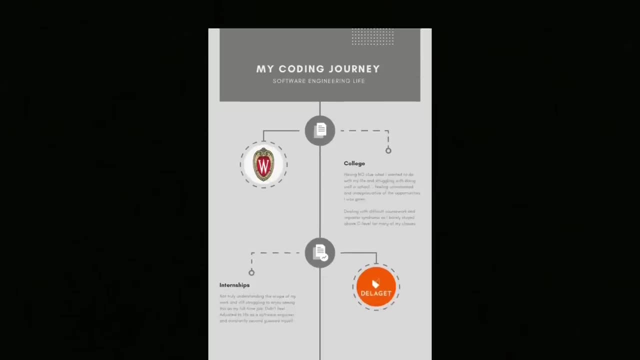 Target. At that point I hadn't even been in the business for a year and a half. I was on my way point. I had a little more confidence in my interviewing skills, since I had now worked for over a year as a software engineer. Now, this is where everything changed. I went through. 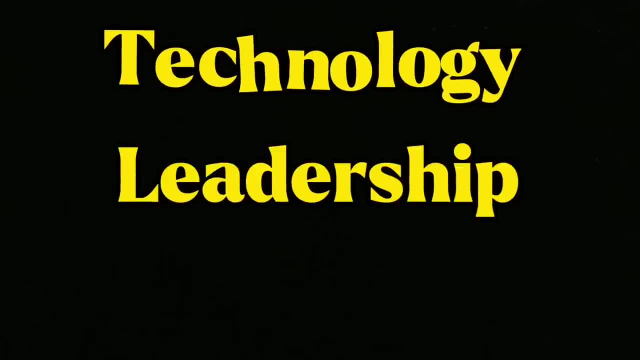 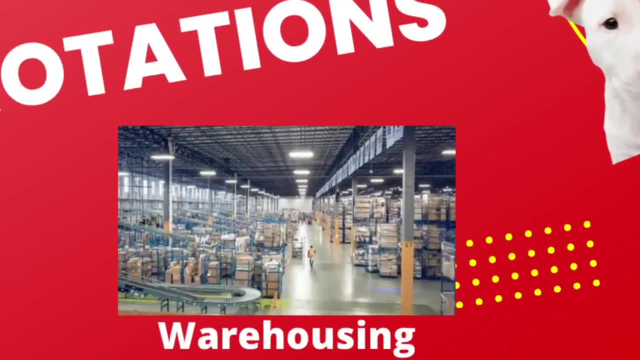 a program called the TLP Technology Leadership Program. that gave me a chance to do two six-month rotations on different teams, kind of like two internships, and then choose a final placement at the end of the year. It was during this time that I learned the concept of the growth mindset. 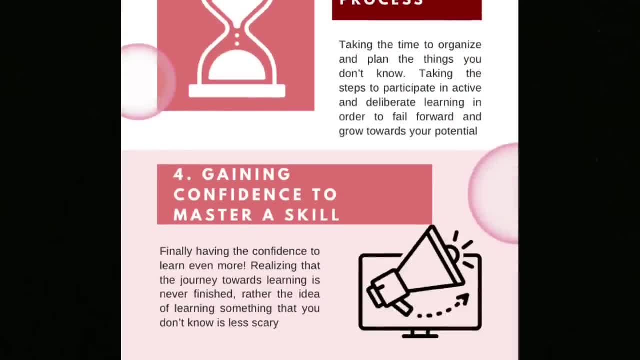 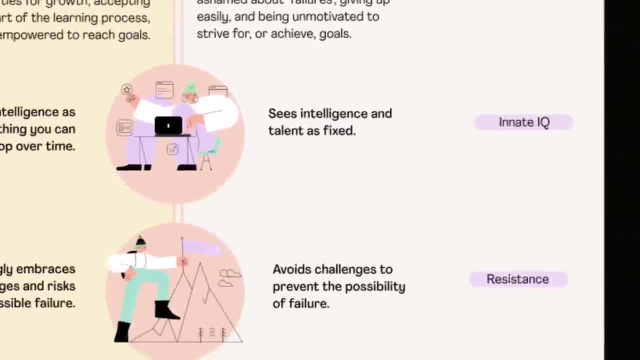 Now, a growth mindset is usually contrasted with a fixed mindset. A fixed mindset just means that you and I have a fixed innate ability, natural abilities when it comes to a profession and there's not much room for variation or growth. But with a growth mindset, everyone starts at zero. 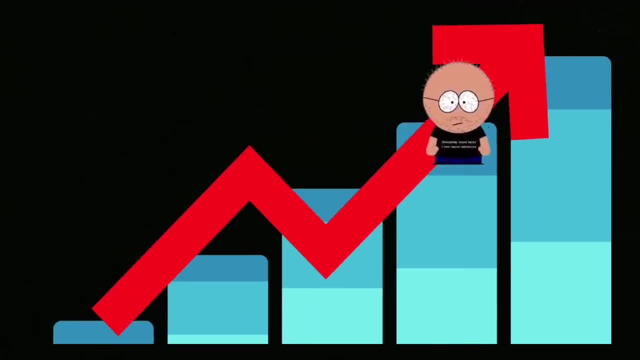 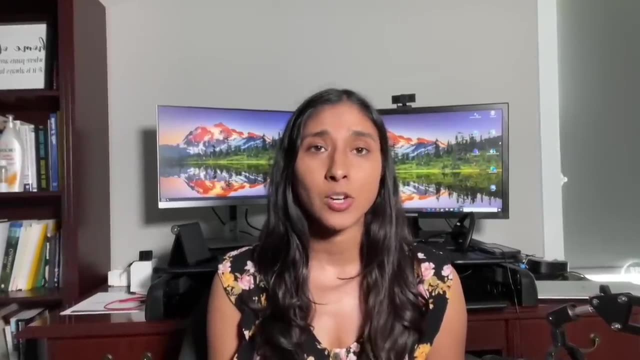 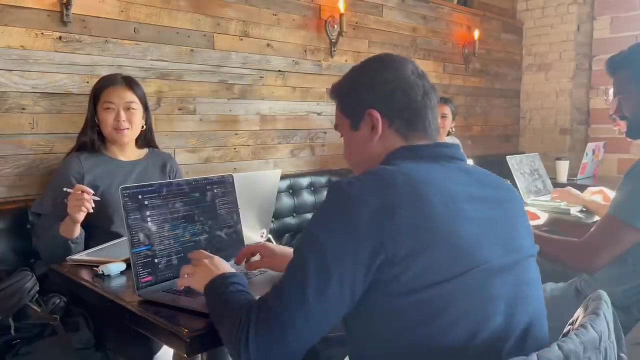 and must learn and fail in order to understand a new concept. At Target, I was told that I was given the room to learn and grow without much pressure, to be insanely productive in my first year on the job. Instead of expecting immediate quantifiable results, it was made clear that we, the TLP-ers in the program, were there to learn. 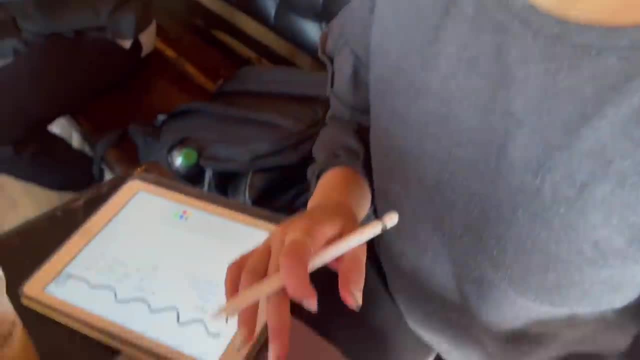 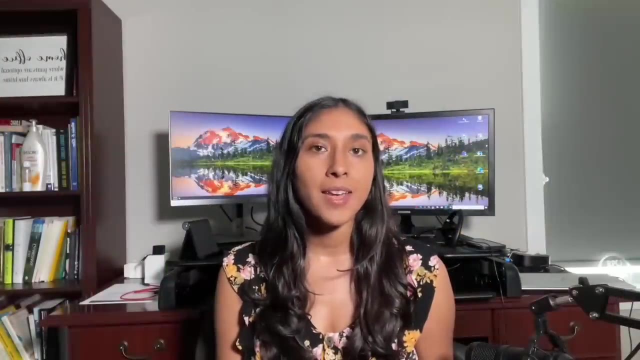 as much as possible so that we could be better engineers in our final placement. As soon as I was given permission to switch my mindset to how can I prove my value to this company, into how can I learn as much as possible, I was finally able to let go of my fixed mindset and realize that, being 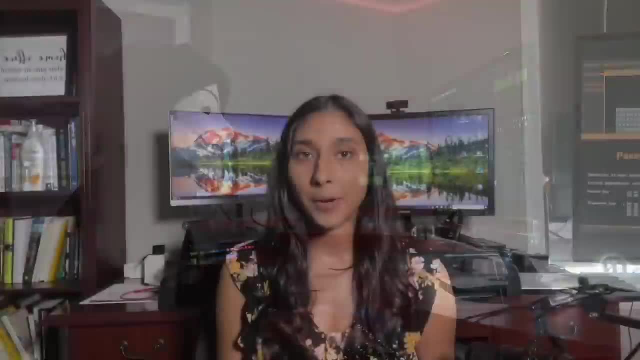 a good coder didn't mean having a natural talent for coding. It meant accepting that everyone sucks at coding. in the beginning, I was able to learn as much as possible and realize that being a good coder is a really beautiful and effective way to become a master of your skills. so if a little 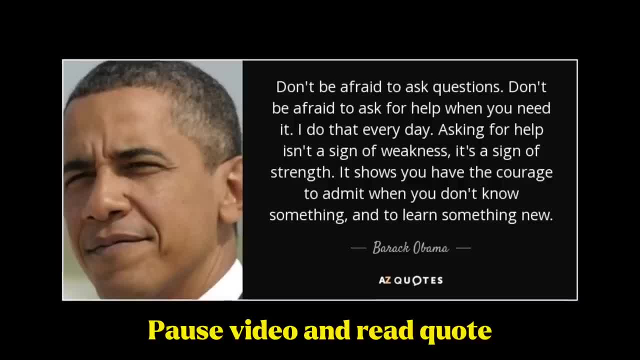 bit of the world and the world does work for you. then you can actually learn by learning. In fact, this is what I found just as interesting to me: You think it's okay to ask stupid questions about something, and it's okay to ask stupid questions about something. In fact, stupid are the. 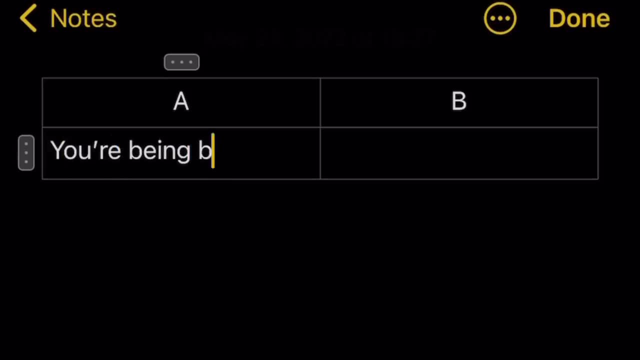 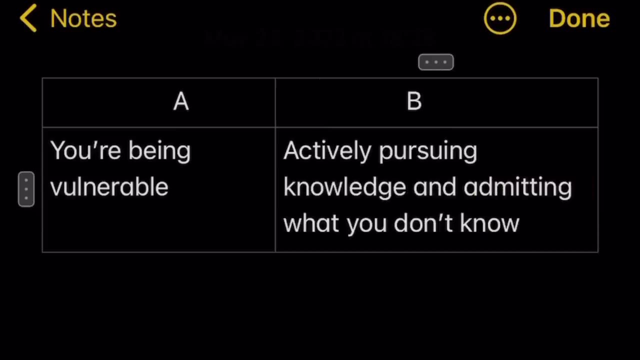 questions A, you're being vulnerable enough to admit to yourself that you need something to learn by. and. B, you're actively pursuing knowledge and learning from it, rather than pretending that you know something already. I always thought that these companies hired me for the knowledge that I had. 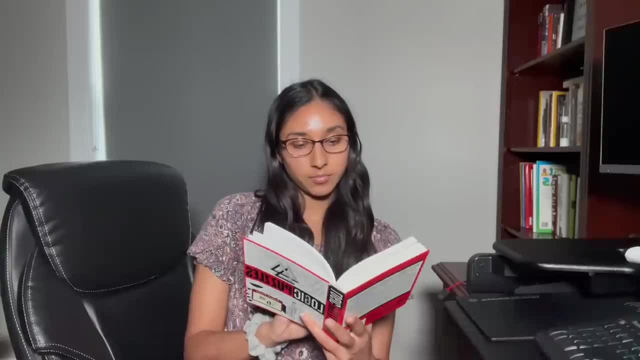 but rather they were hiring me for the potential of what I could learn and then bringing out my own expertise and knowledge. It was just the opposite, It was true. It was so much easier for me to live bring to the table afterwards. So, equipped with this new mindset, I went into every meeting with 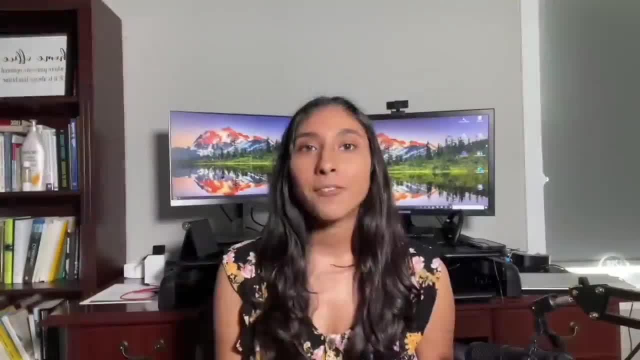 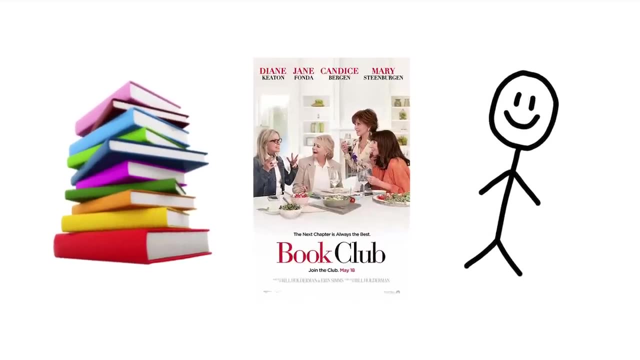 curiosity and a lust for learning something new. It was my final placement where I finally met an amazing mentor that was able to further instill this love for learning in me. We had a coding book club where we would read a chapter of The Joy of Kotlin every week and discuss our learnings. 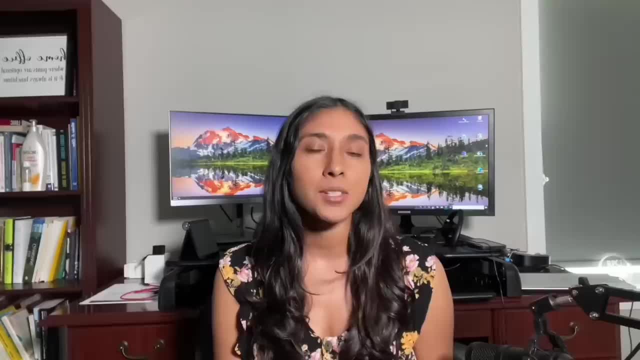 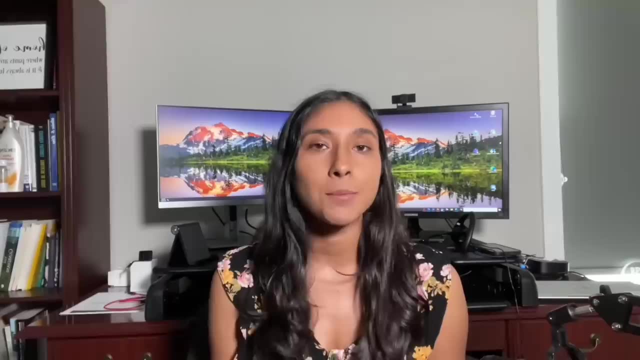 We would meet with other TLPs and eventually my own mentees, to experiment and try out different variations of a problem we were trying to solve for the sake of learning something new and potentially optimizing our solutions. We were told to take our time and truly try to. 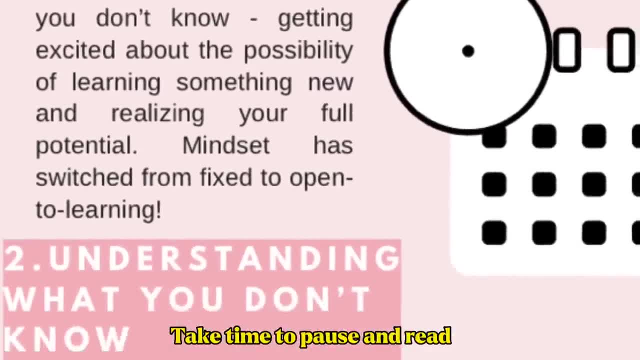 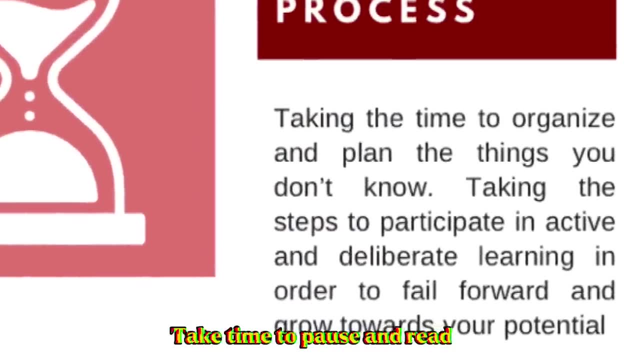 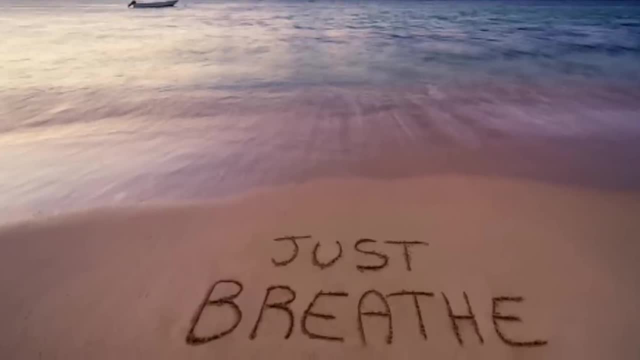 understand the fundamentals instead of just finding the cookie cutter solution to a cookie cutter problem. This room for growth and learning is where my love and competence for coding skyrocketed. I was finally becoming really confident in my ability to code, mostly because I was just giving room to breathe and learn without any pressure. Eventually, I set my sights. 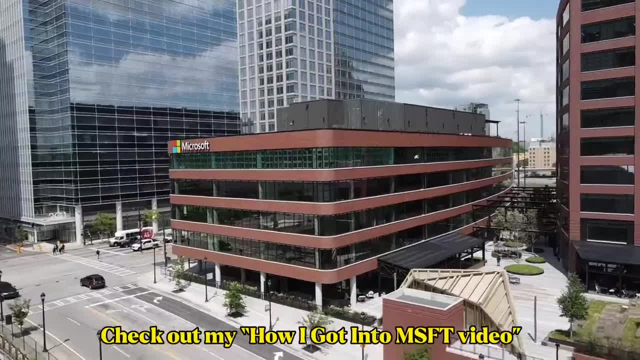 even higher with newfound knowledge and landed a job at Microsoft, a company that I was passionate about. I had a lot of fun doing my job at Microsoft and I had a lot of fun doing my job at Microsoft, but I also had a lot of fun doing my job at Microsoft. 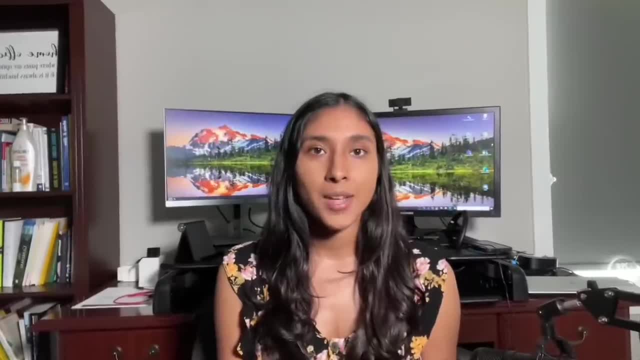 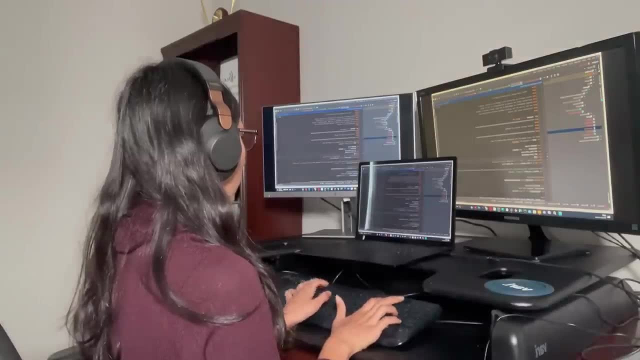 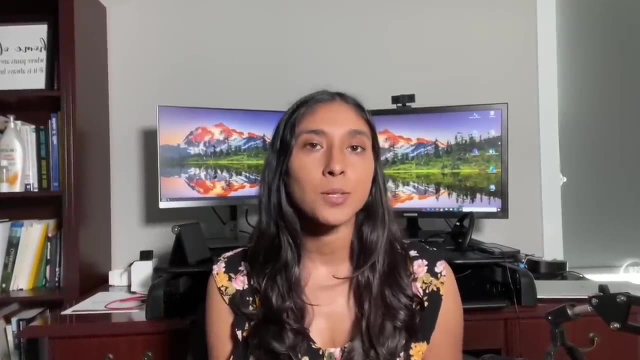 that 18-year-old me never would have imagined getting into. Thankfully, I still feel the same push to grow and learn the psychological safety net in order to eventually become a more productive engineer. Sure, I'm using a different language, framework libraries etc. but I'm still given the room to breathe and 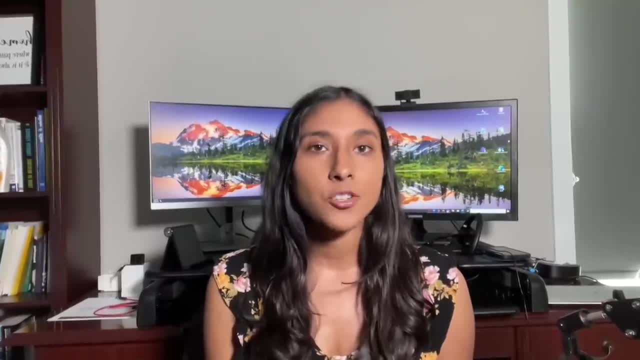 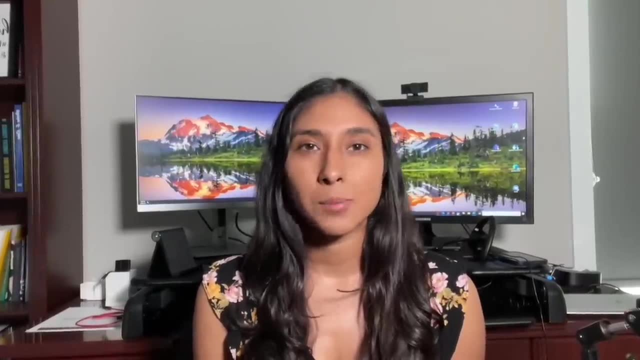 learn, so that productivity becomes a consequence of the potential that I've been given room for, rather than the priority that many companies seek. The whole point of this long-winded way of explaining my journey to coding is to tell you that it gets better. I know it's hard at first and sometimes it can be. 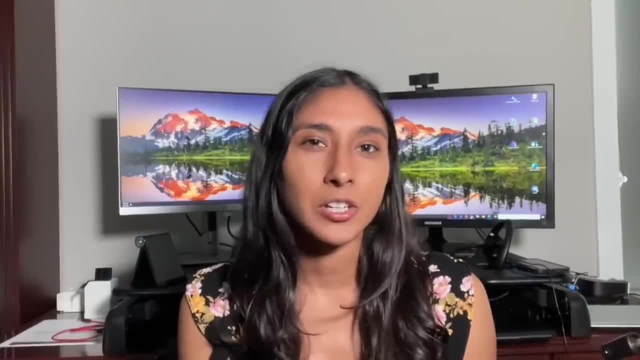 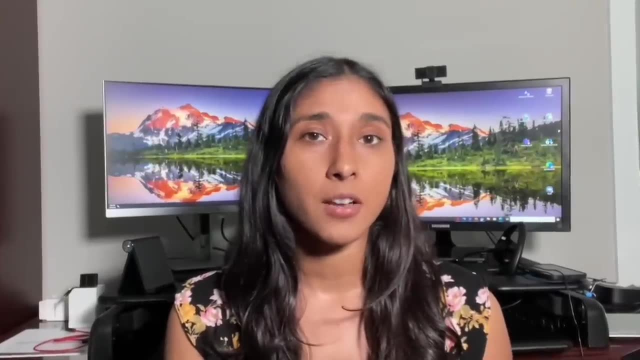 intimidating to see people that may come off as naturally good, but I'm telling you, there's a place for everyone at this table. If I can do it, so can you. All it takes is a little faith in yourself and, honestly, just being okay with starting.